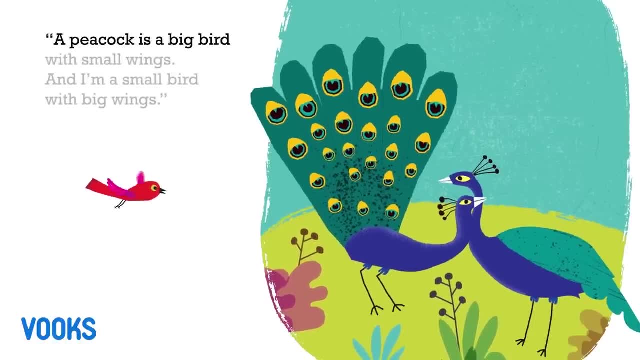 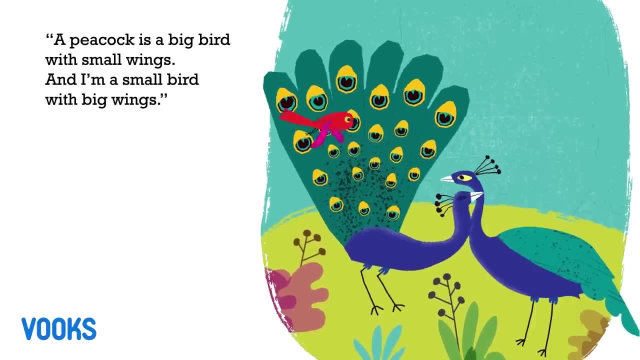 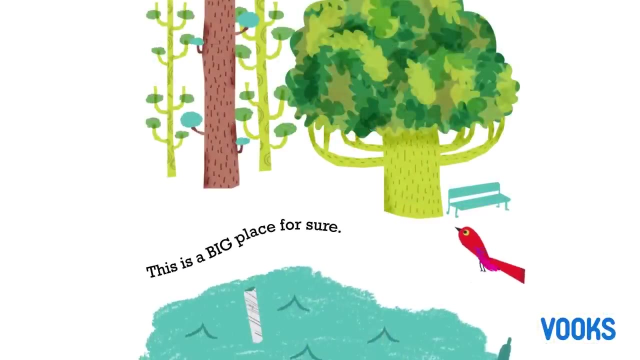 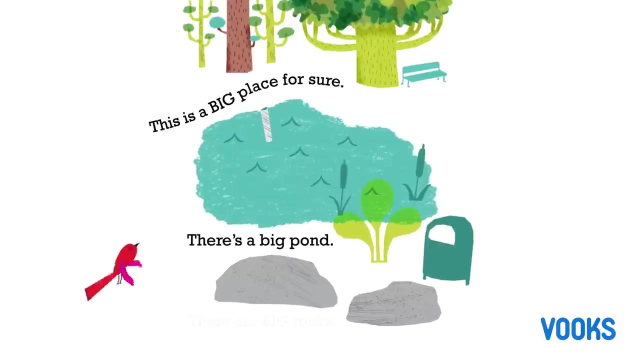 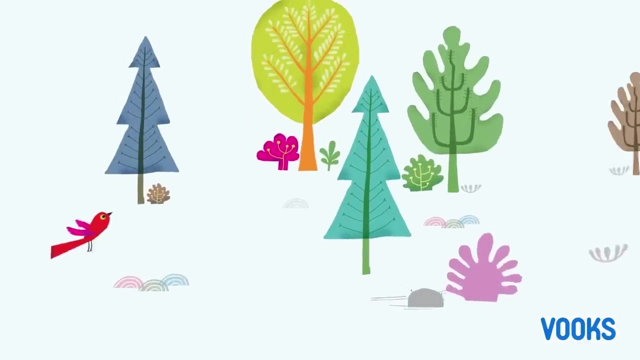 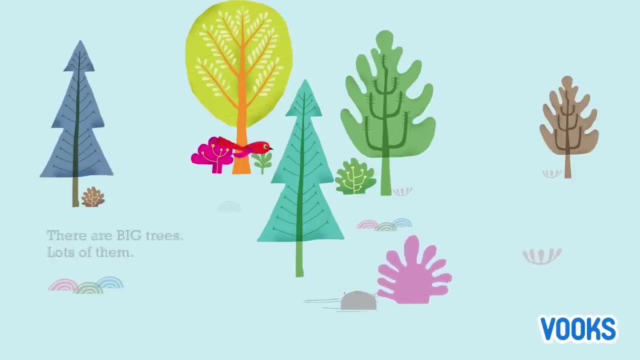 A peacock is a big bird with small wings and I'm a small bird with big wings. This is a big place, for sure. Big trees, Big hippo, Big rock, Big tree, Big tree- Everybody loves big trees. This is a big place, for sure. 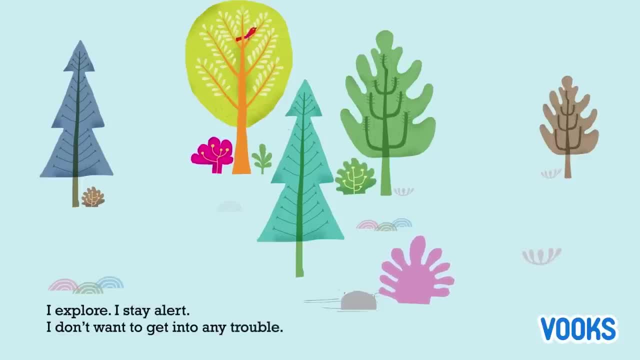 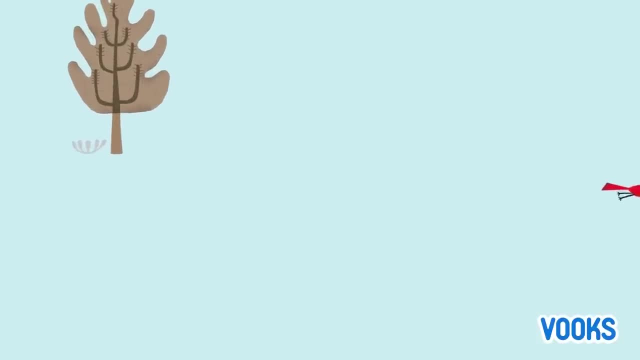 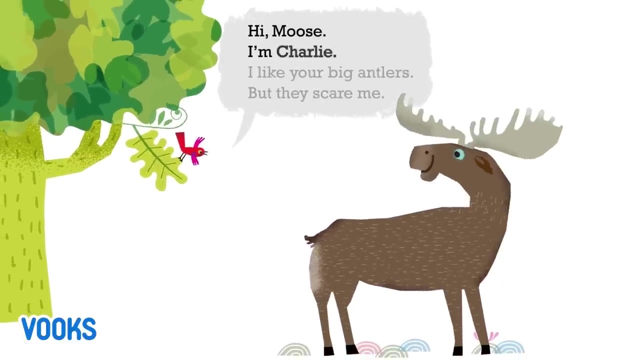 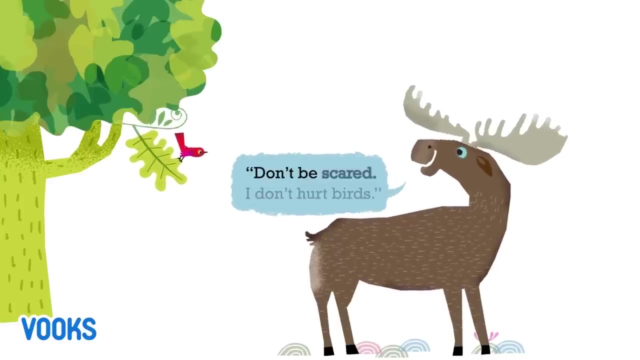 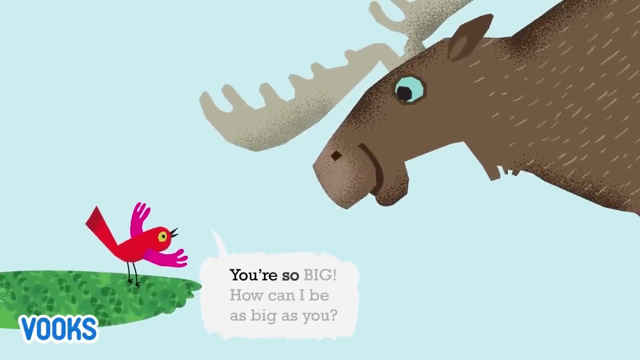 Stay alert. I don't want to get into any trouble. Hi Moose, I'm Charlie. I like your big antlers, but they scare me. Don't be scared, I don't hurt birds. You're so big, how can I be as big as you? 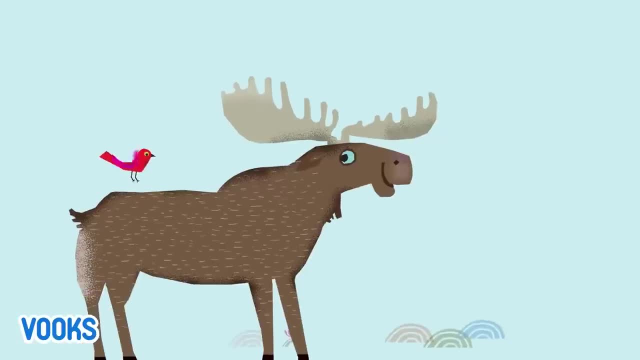 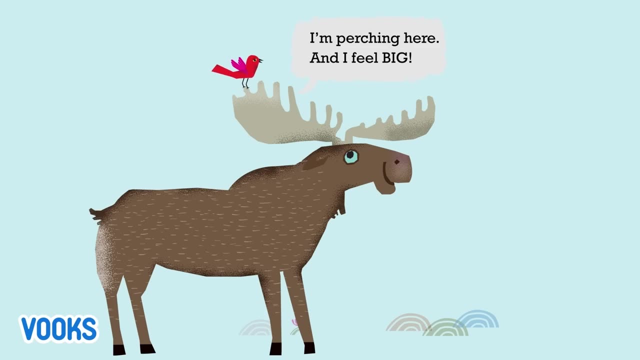 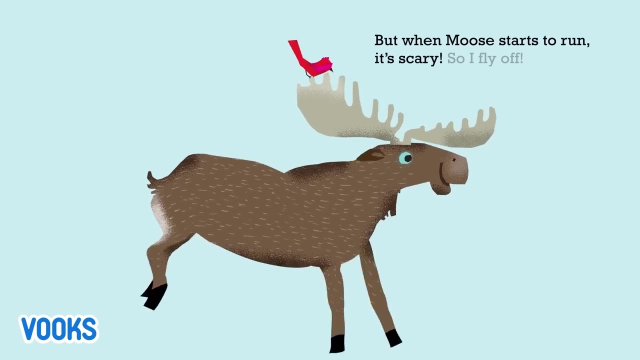 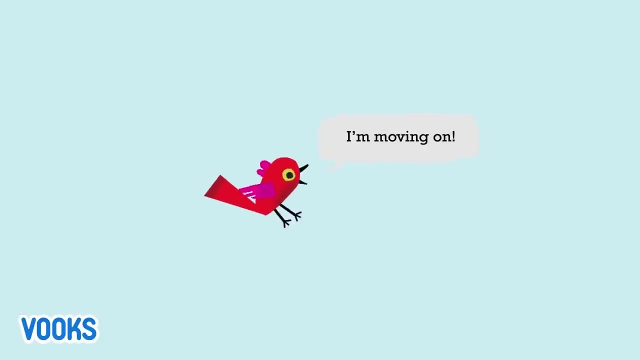 Perch on my antlers. I'm perching here and I feel big Whoa, but when Moose starts to run it's scary, So I fly off. whoa, I'm moving on. I touch down near a pond. 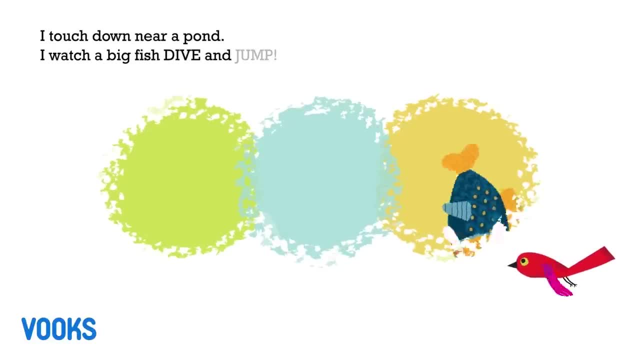 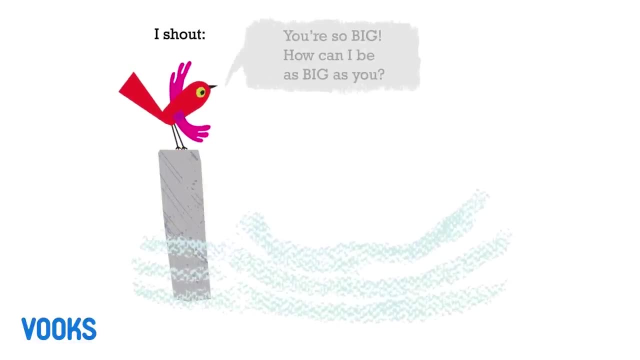 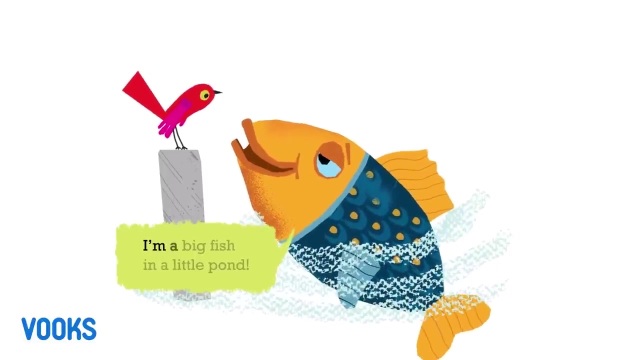 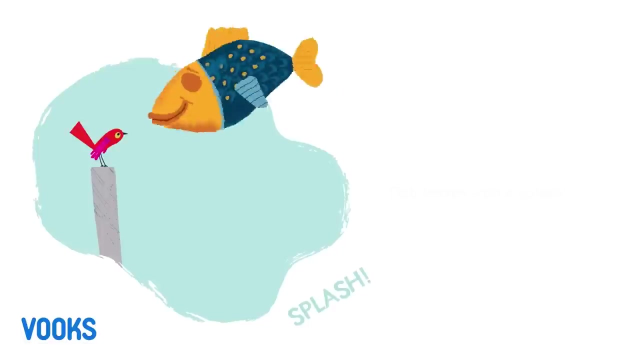 I watch a big fish dive and jump. I shout: you're so big, how can I be as big as you? I'm a big fish. I'm a big fish in a little pond. Splash Fish leaves with a splash Whoa. 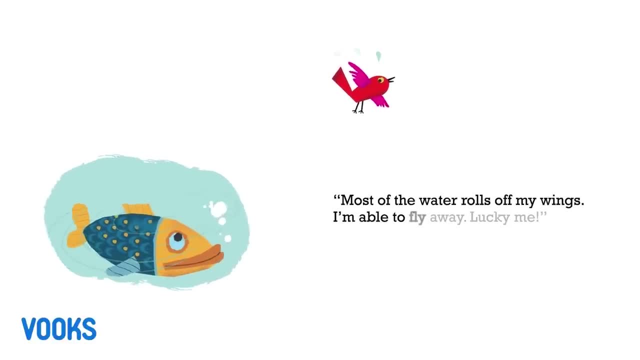 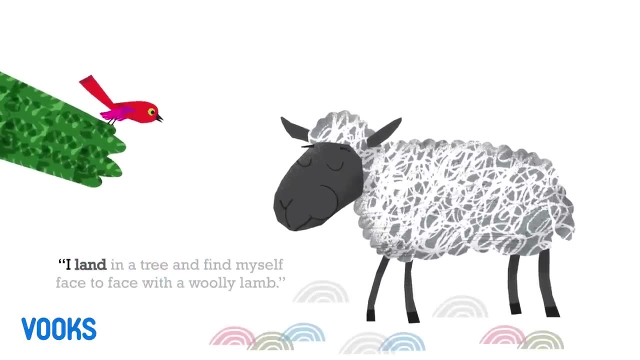 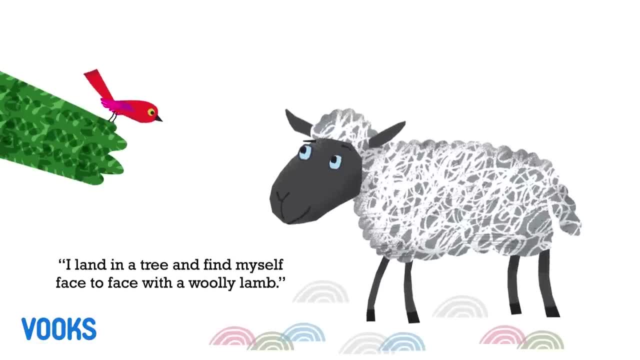 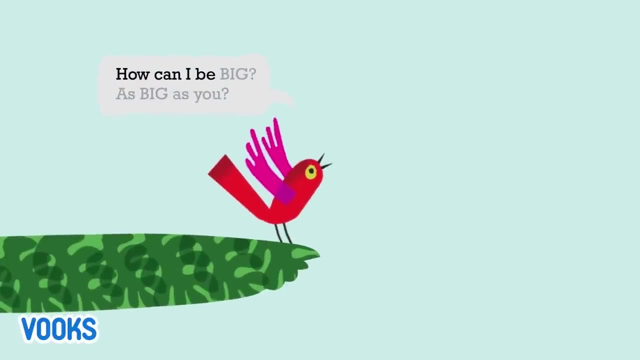 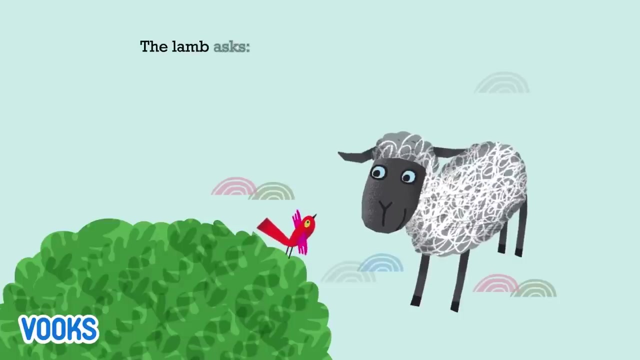 I'm a big fish. I'm a big fish. What can I be big like the Lamb? What can I be big like the Lamb? Hmmm, No answer from the Lamb. How can I be big, as big as you? The Lamb asks: what do you want to be big? 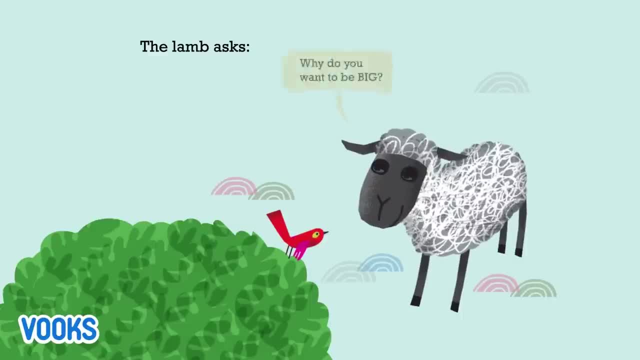 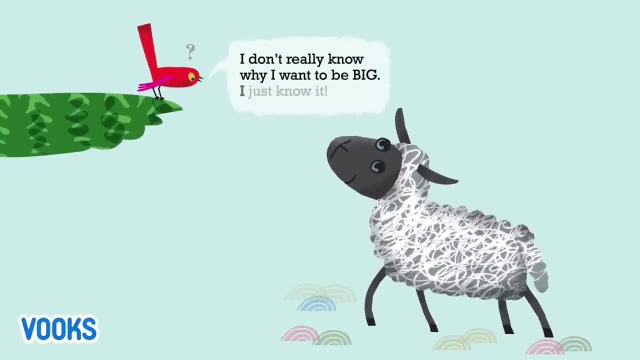 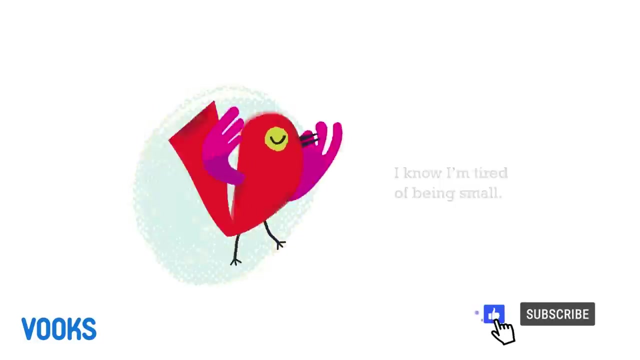 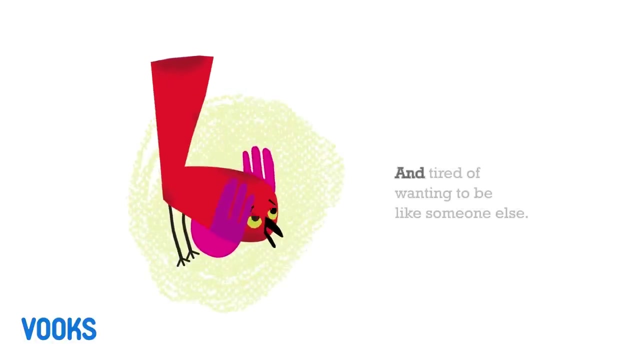 The Lamb asks: why do you want to be big? What can you do, Dak? twenty-six inches high, 雨 40.. I don't really know why I want to be big, I just know it. I know I'm tired of being small. I know I'm tired of being scared and tired of wanting to be like. 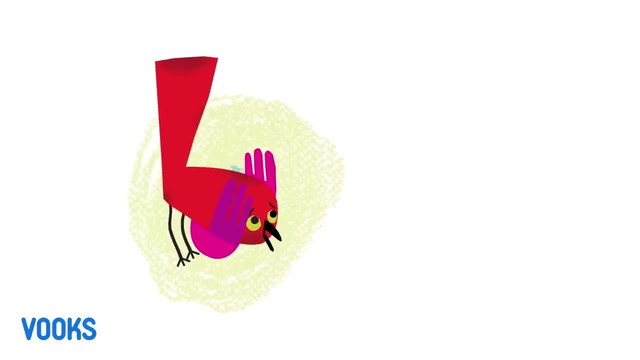 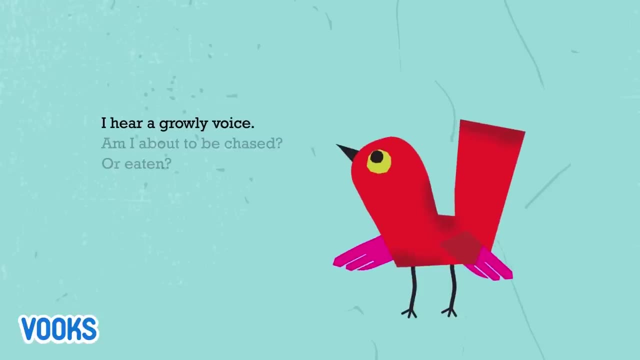 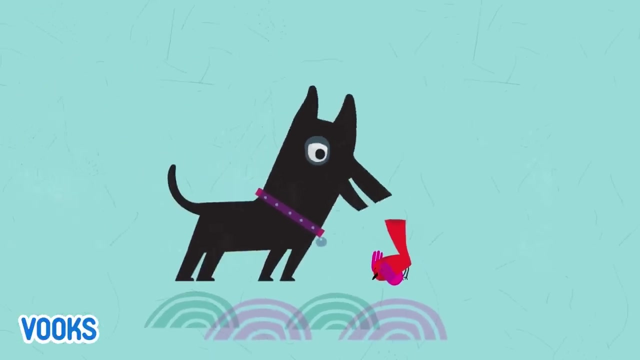 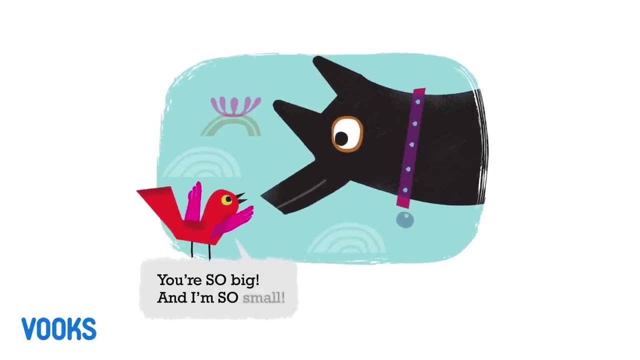 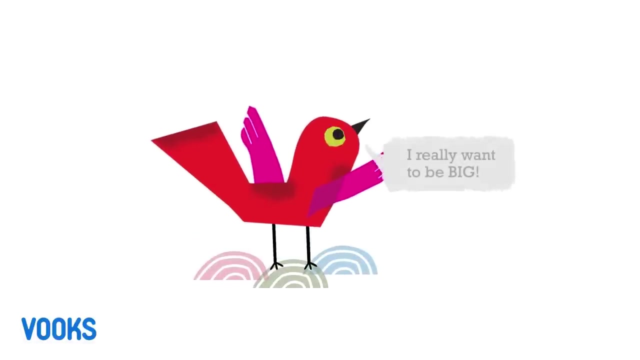 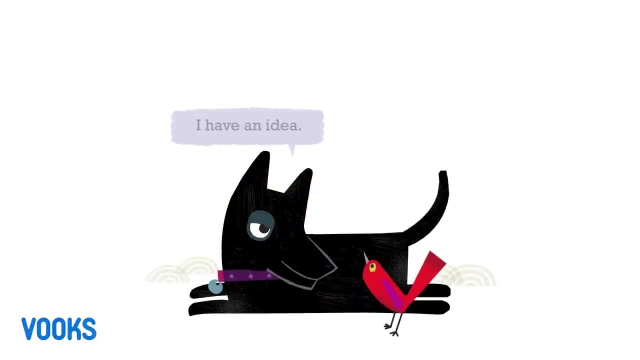 someone else? I hear a growly voice. am I about to be chased or eaten? don't be scared, I won't hurt you. how can I help you? you're so big and I'm so small. I really want to be big. I have an idea. I'm listening. 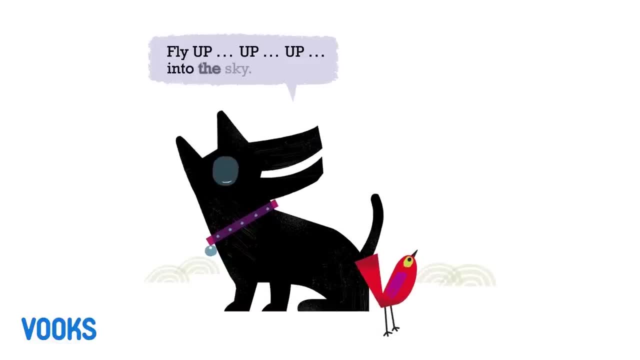 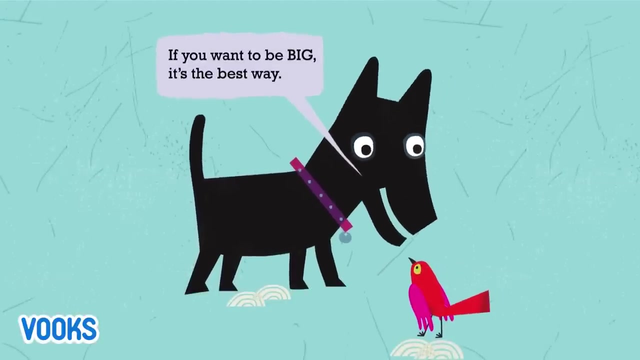 like up, up, up into the sky, fly as high as you can, then look down. I really want to be big. I have an idea. I'm listening, I'm listening. fly, up, up, up into the sky, fly as high as you can, then look down. that's scary. it will not be easy. if you want to be big, it's the best way, okay. 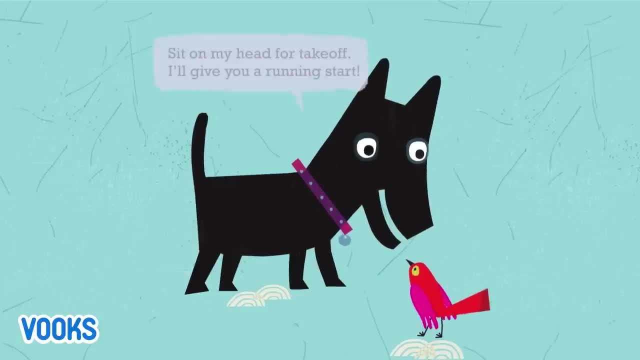 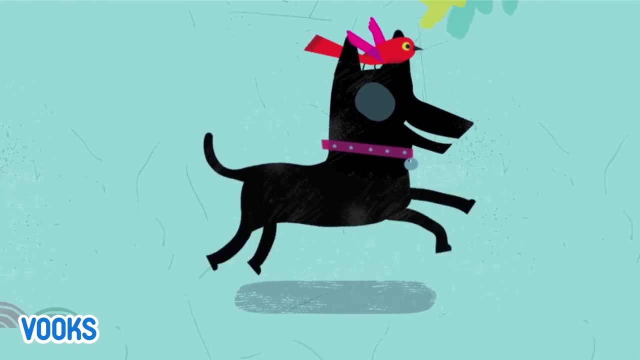 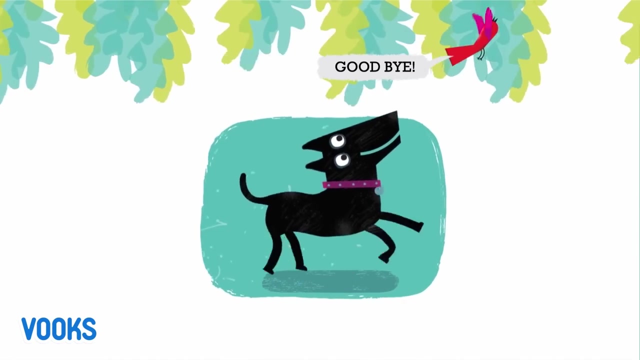 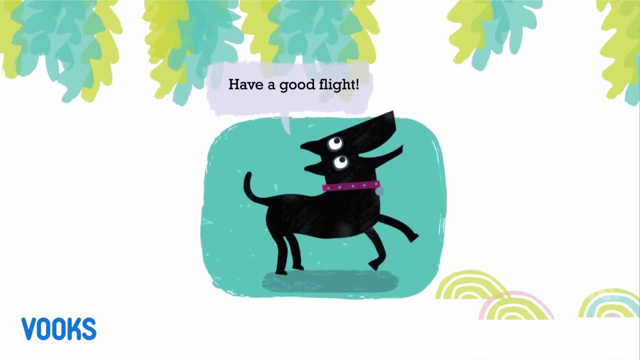 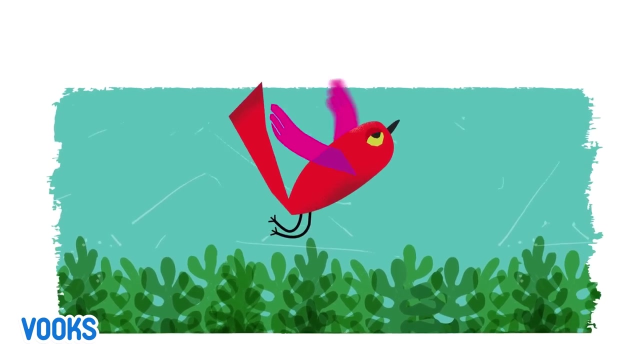 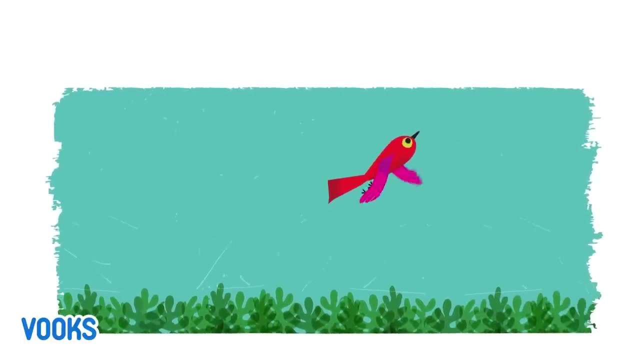 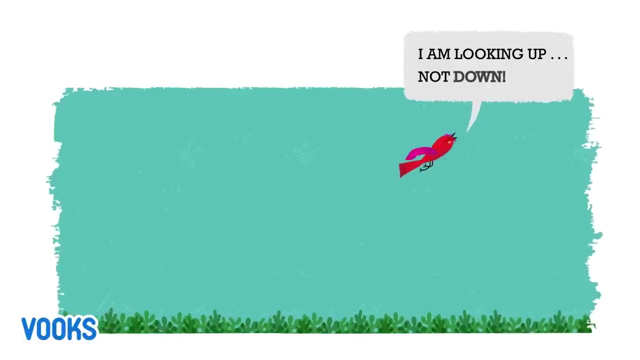 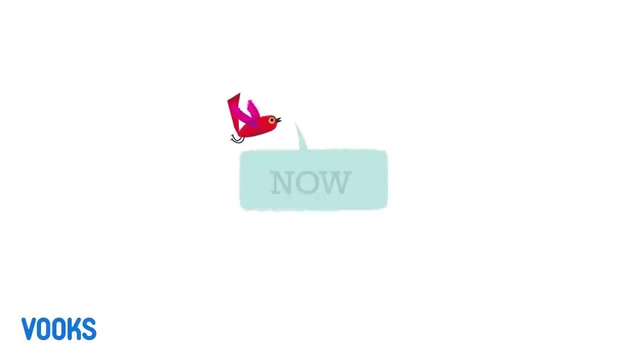 I'll try. sit on my head for takeoff. I'll give you a running start off. you go off, you go go, goodbye, have a good flight. I'm flying, I'm flying. I'm flying higher and higher. I'm flying higher and higher. I am looking up, not down. Now I am ready, ready to look down. 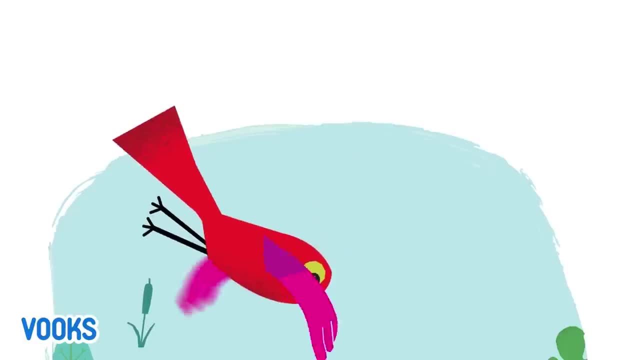 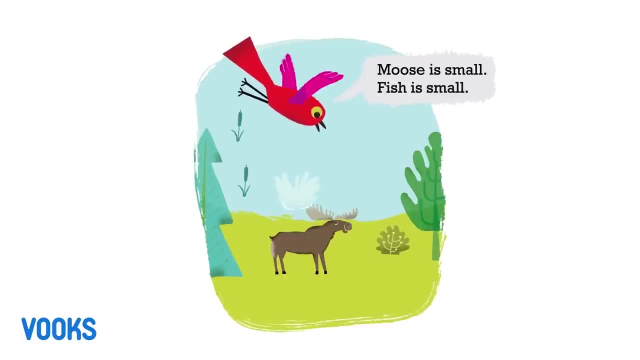 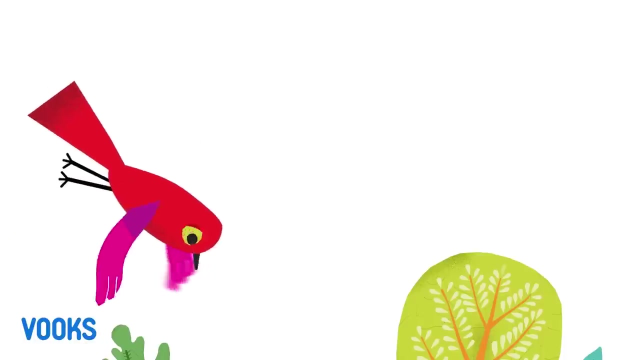 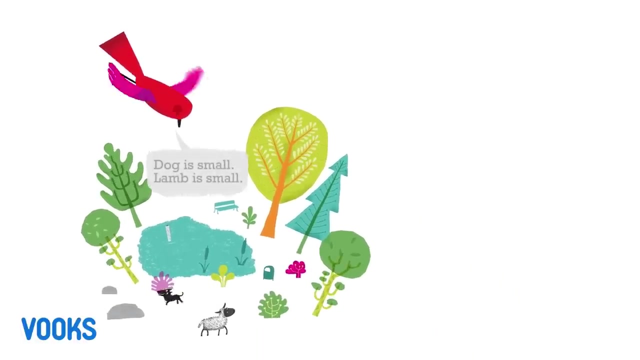 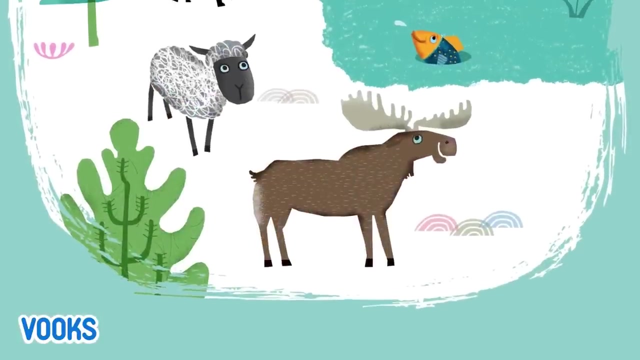 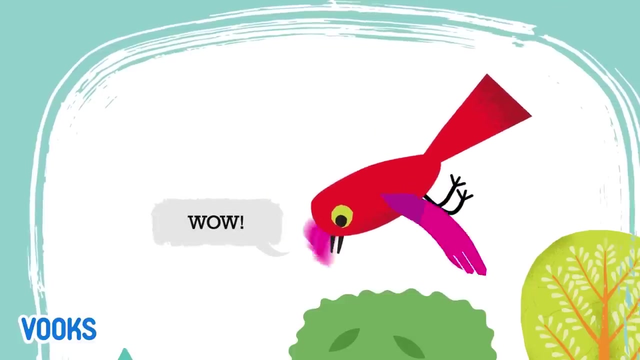 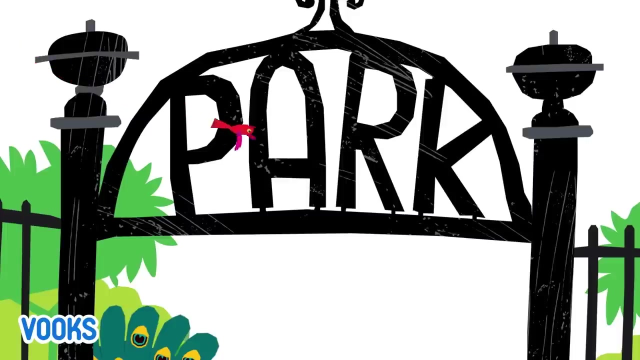 I'm looking down. Moose is small, fish is small. I am big, bigger than everyone. I am big, bigger than everyone. I am big, bigger than everyone. Dog is small, lamb is small, Everything is small. Wow, I am Charlie, a small bird. 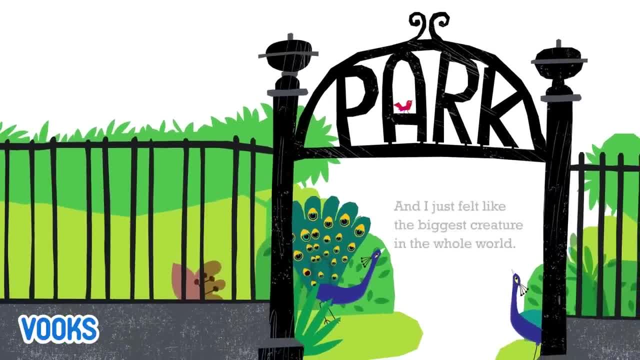 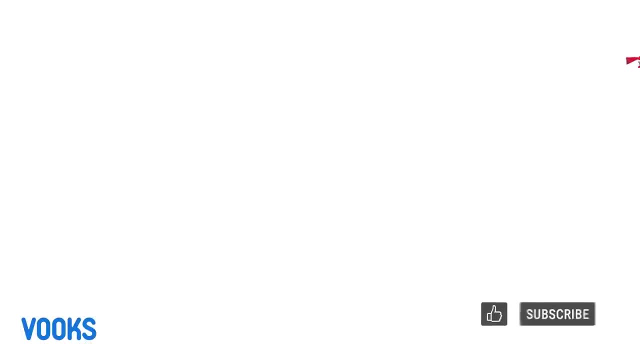